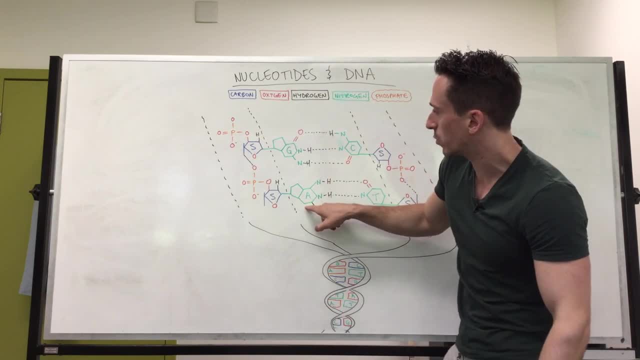 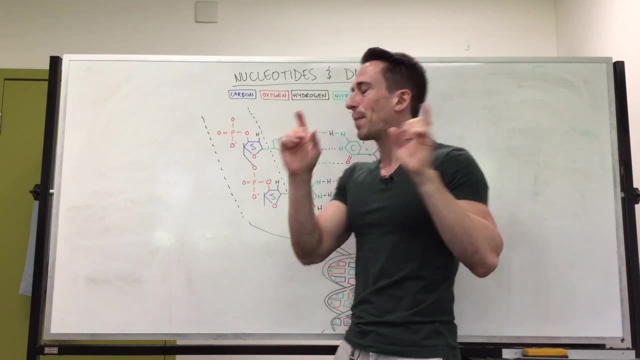 two rings. These two rings link together, as you can see, with this one here and this one here. So that means that that is a nucleotide nucleotide, nucleotide, nucleotide. So if we break them up into those of the double rings, they're called purines. So those nucleotides, 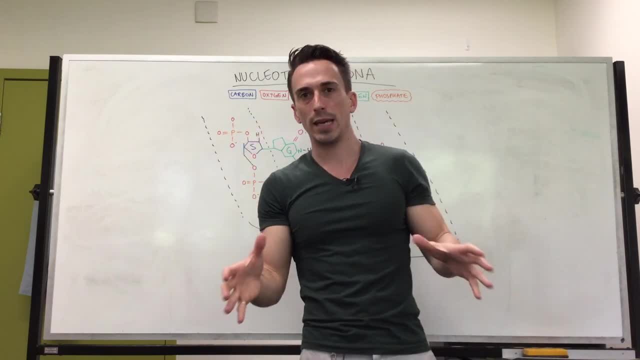 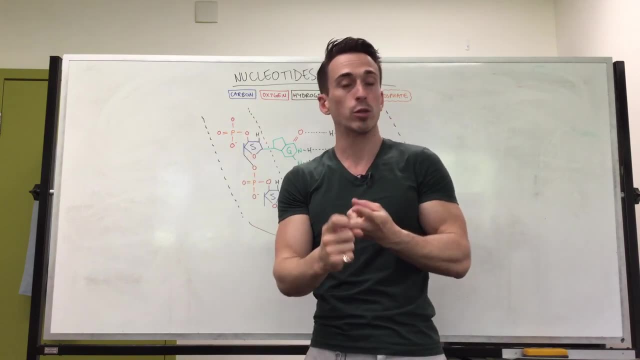 are termed purines, Those of the single rings, they're called pyrimidines. Now, the other thing is this: why do we have nucleotides? We've spoken about with carbs they're for energy, proteins they're for multiple functions and structure, and fats also for energy storage. 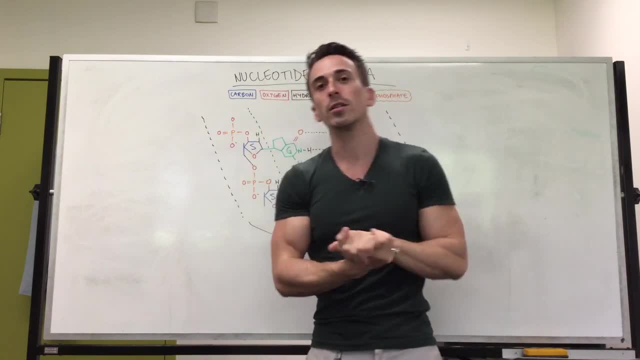 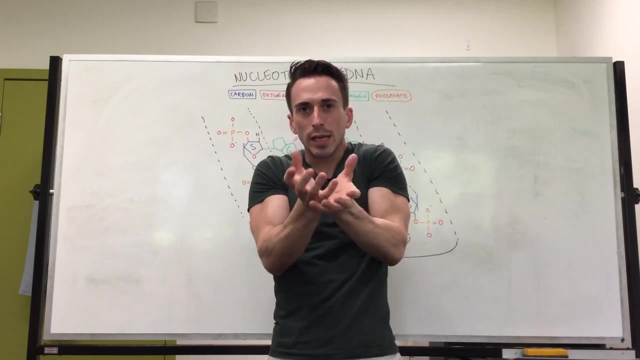 and also for protection as well. But what about nucleotides? Nucleotides are there because they make up our DNA. Now, our DNA is our genetic material, sits within the nucleus of our cells and it basically is like the blueprint for our life. It turns into genes. 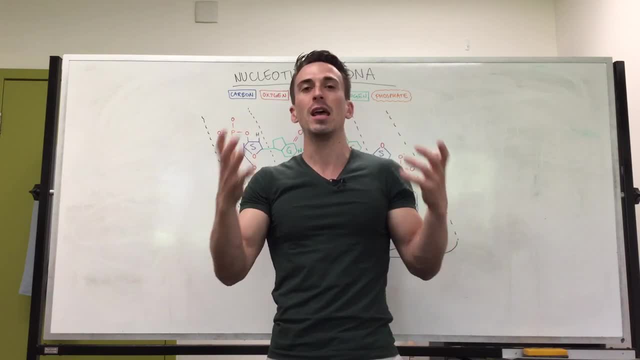 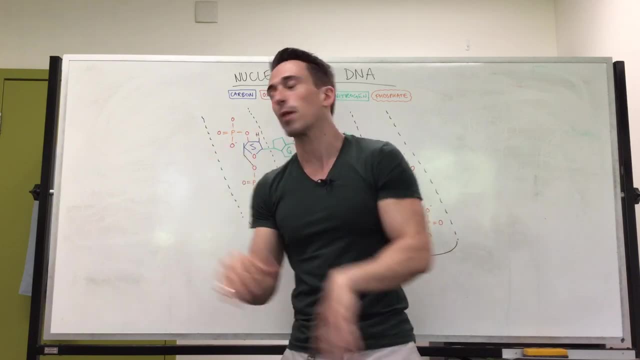 genes turn into proteins. proteins have a function and our body is made up of proteins function. So let's have a look and see how nucleotides make up proteins. So here's a nucleotide. here, this nucleotide you can see I've put a G in one of those nitrogen. 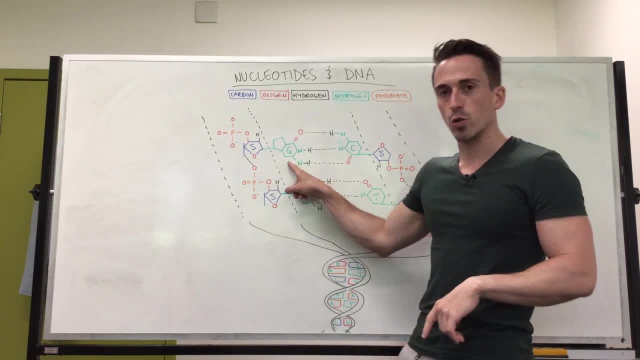 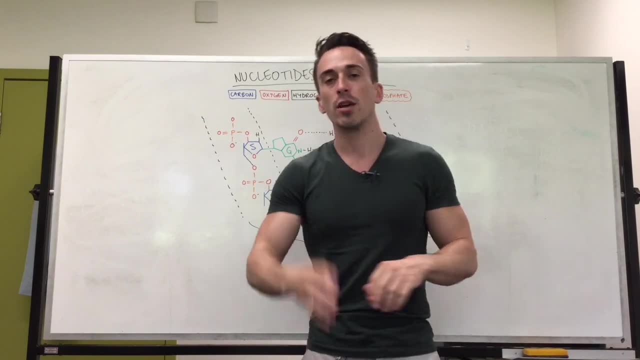 based rings, that's called guanine. So this nucleotide's guanine, This one with an A is adenine, this one with a C is cytosine, this one with a T is thymine. So there are these four nucleotides. in actual fact there's five. the fifth one is called uracil, which is very 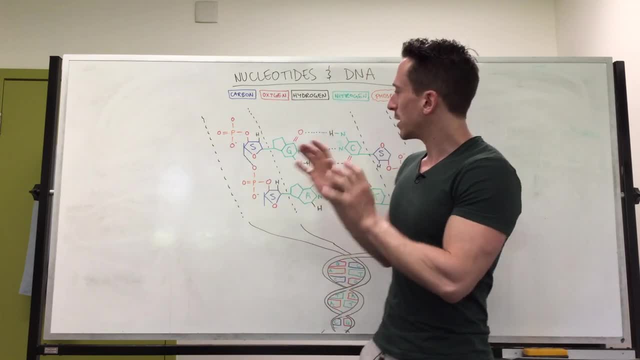 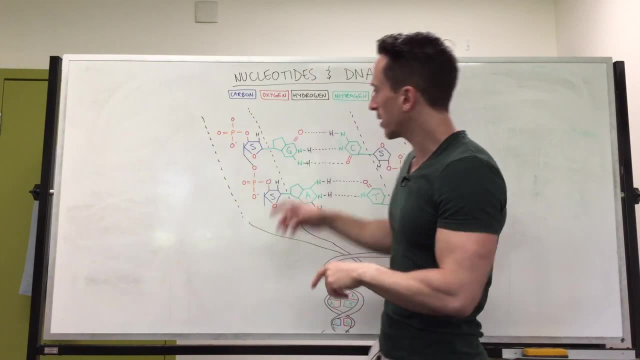 similar to a thymine. We'll talk about that in a future video. So these nucleotides are G an, A, a C and a T. In order to make DNA, they need to be bound to a couple of other things. First thing they need to be bound to is a sugar molecule, So you can see each 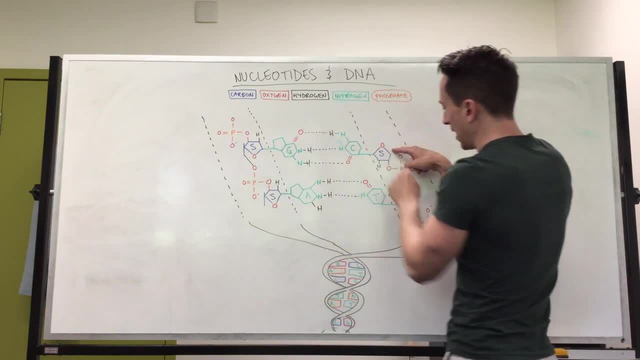 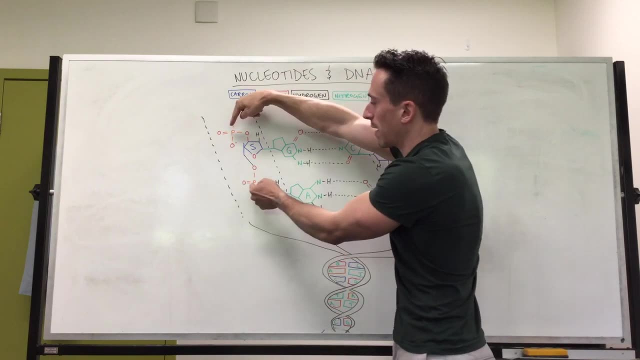 of them are bound to a sugar molecule that I've denoted here with an S. This sugar molecule is very similar to that of glucose. Now, the sugar molecule is always attached to this phosphate molecule, So you can see phosphate, phosphate, phosphate, phosphate, Phosphate. 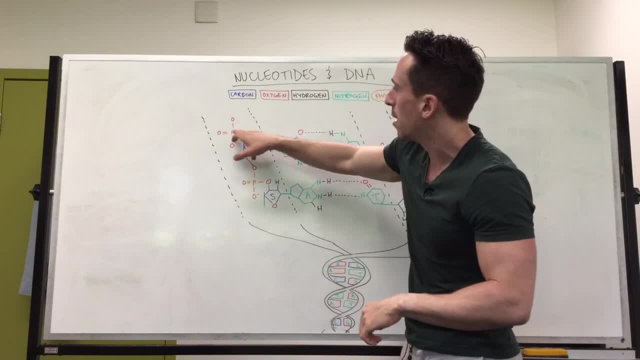 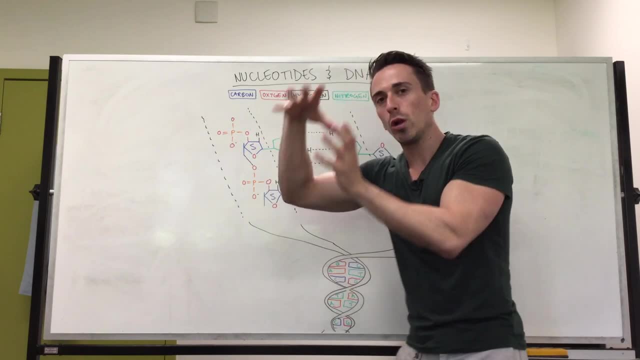 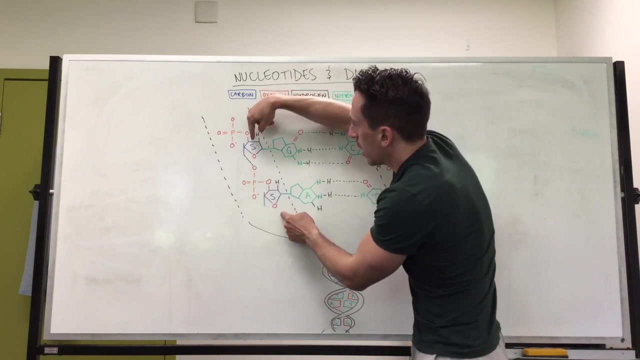 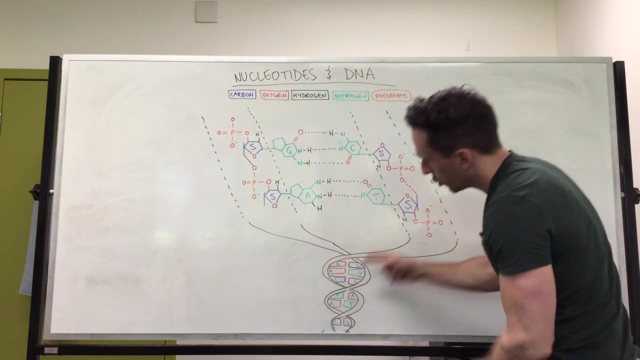 is a PO4- and you can see that there- PO3-. So when we have a look at this, we can see DNA molecules will have a nucleotide, one of the four or five, a sugar and phosphate backbone. so here we go. here's the backbone, which is sugar and phosphate comes together and you can see what will. 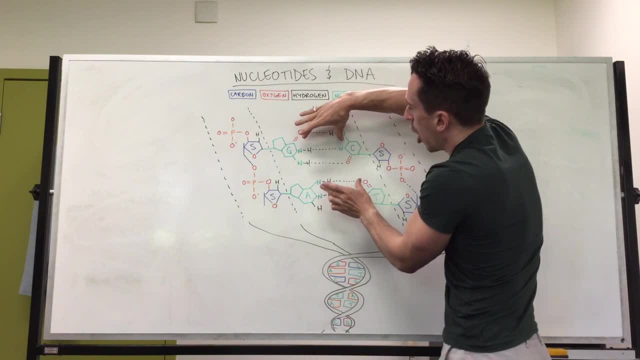 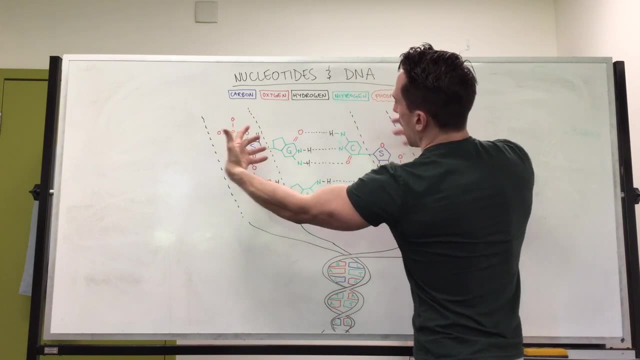 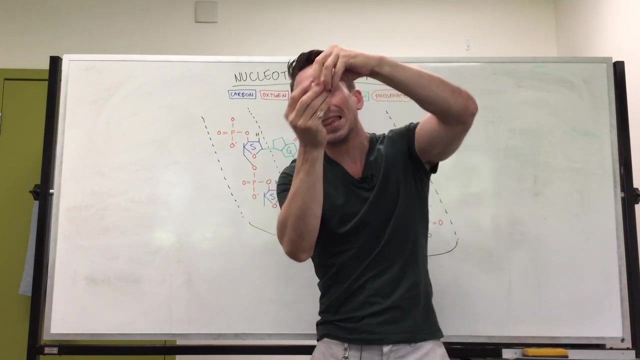 happen because the individual nucleotides make hydrogen bonds with one another. we now have one strand of DNA, another strand of DNA bound together having a conversation and they wrap around into this double helix structure. so it is a linear. that means straight molecule. there's two strands. 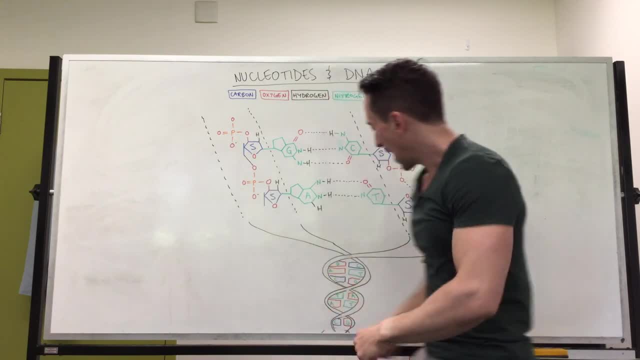 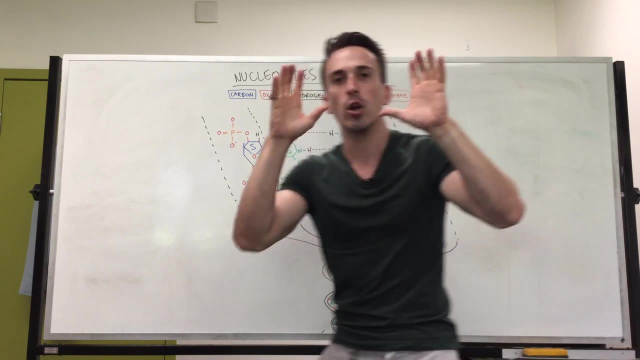 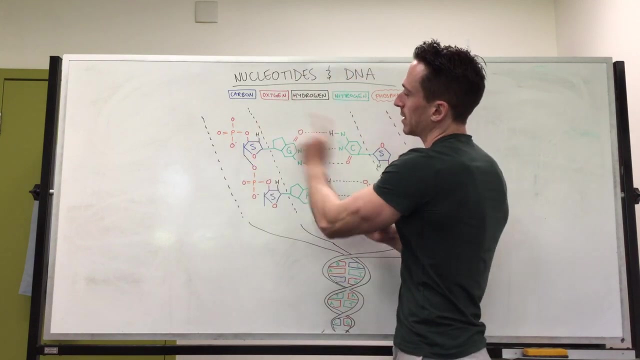 bound together in a helical fashion and it looks like the rungs of a ladder. now those rungs are the conversations that have been had between the nucleotides, and always a G will always speak to a C, that's a guanine. always speaking to a cytosine, they will always. if a C's on this side, will talk. 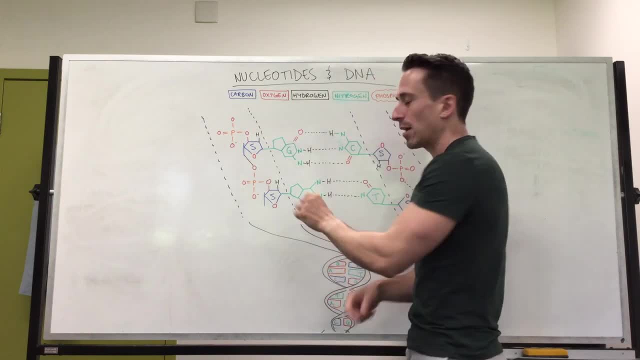 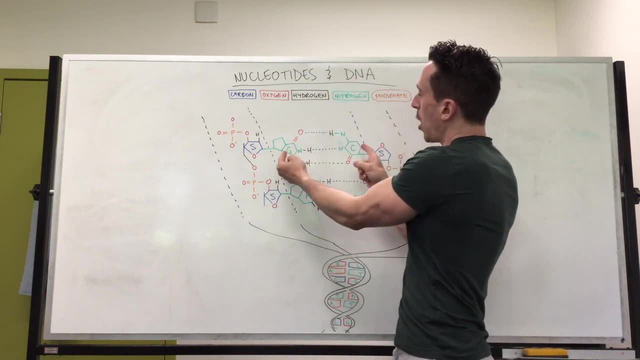 to a G on that side and vice versa. an A which is an adenine will always talk to a C and vice versa to a T on the other side which is thiamine, and vice versa. The G's binding to the C's will always be three hydrogen bonds: always An A talking to a T will. 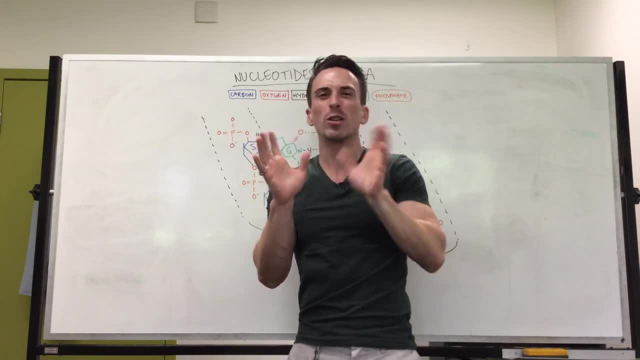 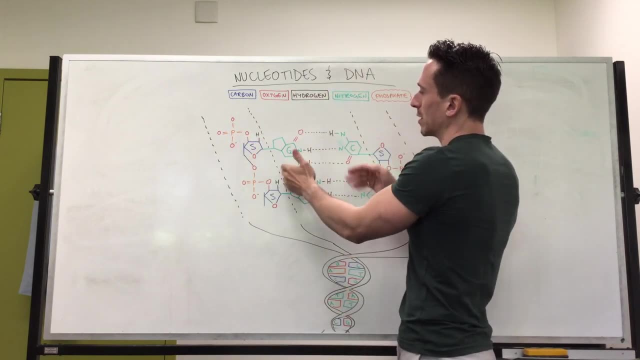 always be two hydrogen bonds. Now, this may not be of too much clinical relevance clinically, but it is when we do scientific research, because it means it's harder to break the bonds between a G and a C and it's easier to break the bonds between an A and a T. Sometimes what we want to do when we do research. 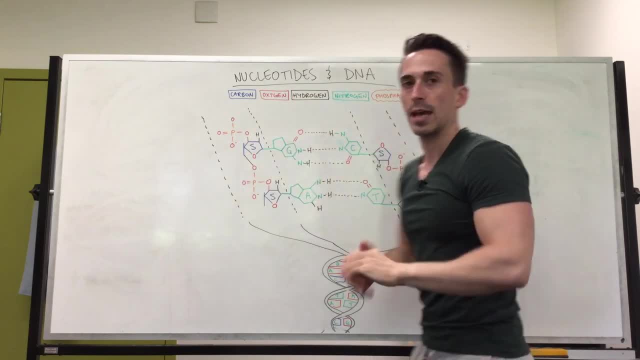 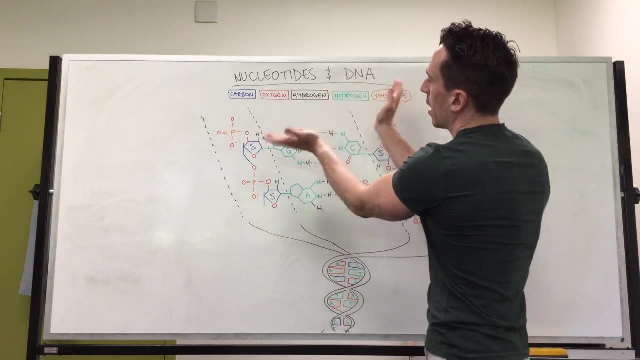 is, we want to make multiple copies of DNA and in order to do so, we need to unravel this DNA. so unwrap it and open it up, and we can do this using temperature. Increase the temperature. it opens it up, but when you've got more G's. 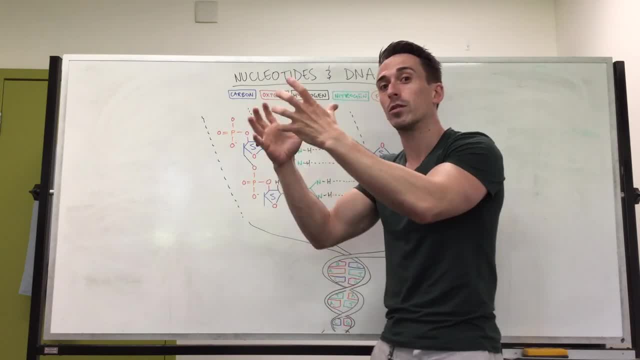 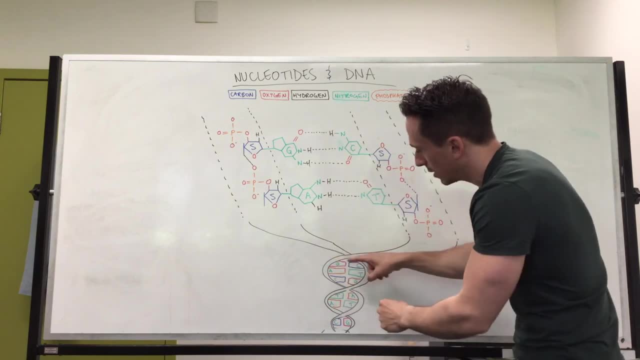 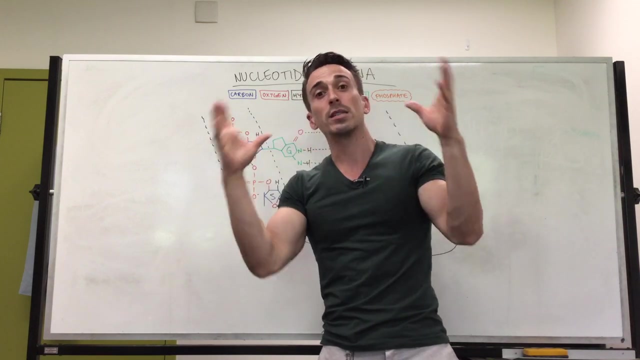 and C's. there's more bonds. the temperature needs to be greater in order to open this DNA up. Okay, now, another important point is, when we have a look at the DNA, you can see that, ultimately, what it comes down to is our DNA is made up of those four nucleotides A, G, T and C, in what seems to be a random order.